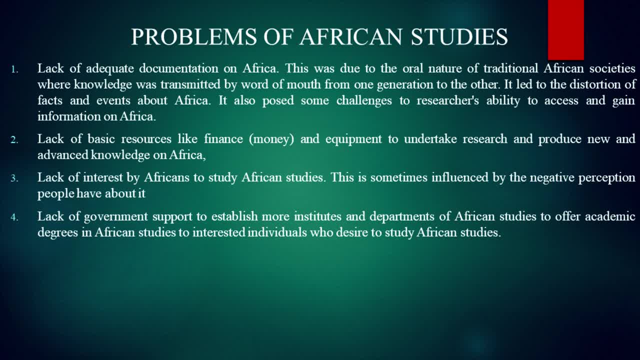 The second was the role of the Africans themselves. There we highlighted some of the deeds or behaviors of the African people which gave them a bad image both in Africa and outside Africa, And this bad image made Africa seem like a continent not worthy of any academic attention. We also talked about the philosophical arguments. 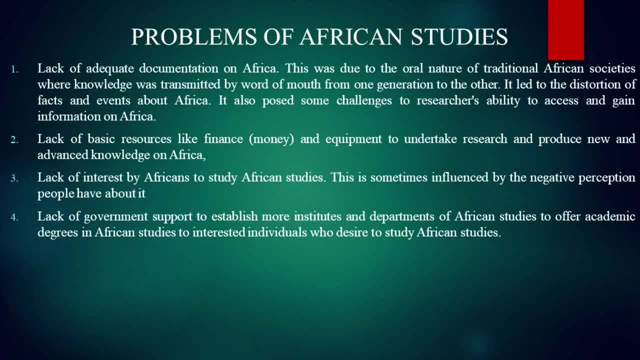 where some early European scholars argued that Africans are an inferior people with an inferior mind, Incapable of producing any intellectual knowledge. The last was the work of the missionaries, which is also based on how the missionaries reported Africans to the outside world. They reported Africa, or the people in Africa, as primitive, barbaric. 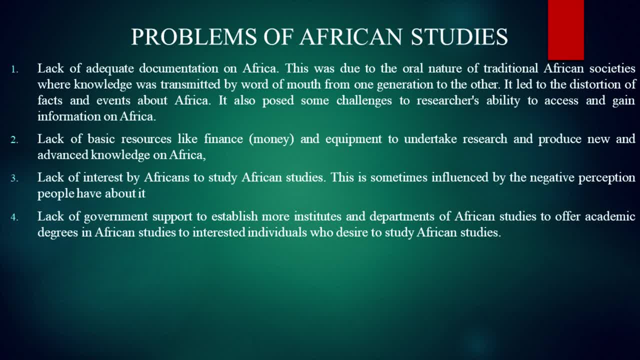 with religion which is polytheistic in nature, With religion whichfon inclination of niemandrep cambio indiet. Wonderful mind. handwriting markens the concept of the authority Who make the religious rawness of may. all these things put together delayed the development of African Studies. we. 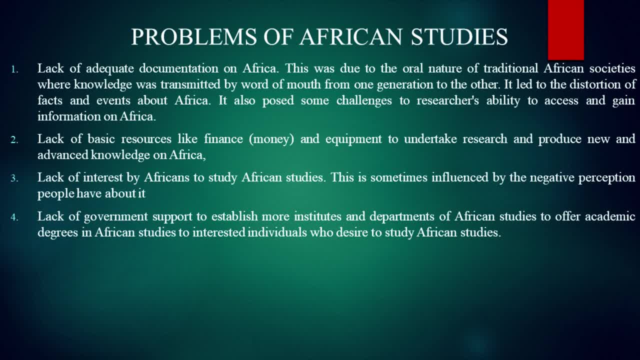 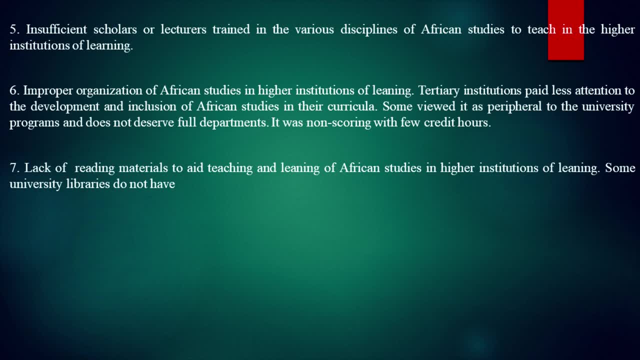 further indicated that some African scholars and to some extent some early Europeans as well, offered counter arguments which eventually led to the establishment of African Studies as an academic discipline, both on the continent of Africa and outside the continent of Africa. we went further to discuss some of the misconceptions about Africa. we said that misconceptions are: 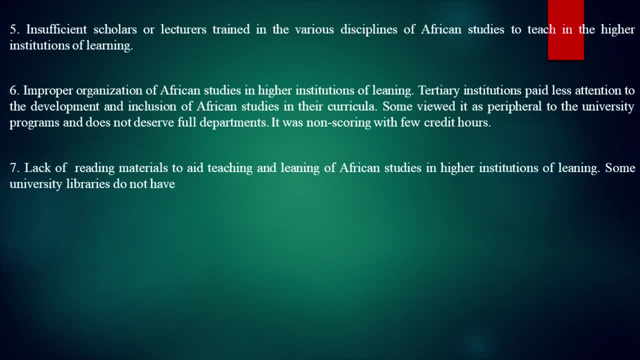 incorrect views, opinions or some false information that are portrayed or given about a person or a group of people with respect to Africa. we studied last week that there are certain misconceptions or certain ideas that have been portrayed. they included the idea that Africa does not have a history, Africans are primitive, barbaric and that Africa 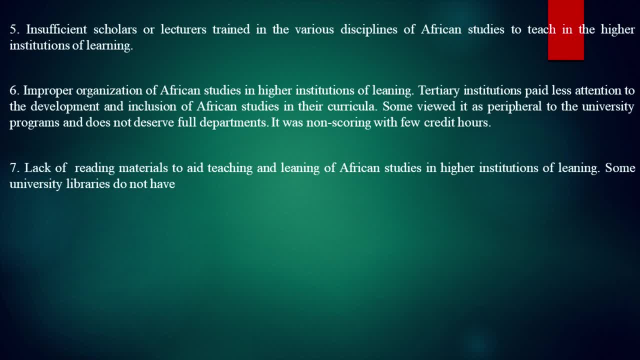 is a continent of crisis, full of corruption, overpopulation and conflict. we further went on to address some of the misconceptions that we found that the African Studies. we further went on to state that there is also a misconception that Africa is a continent or a race. we further went to state that Africans are inferior people. 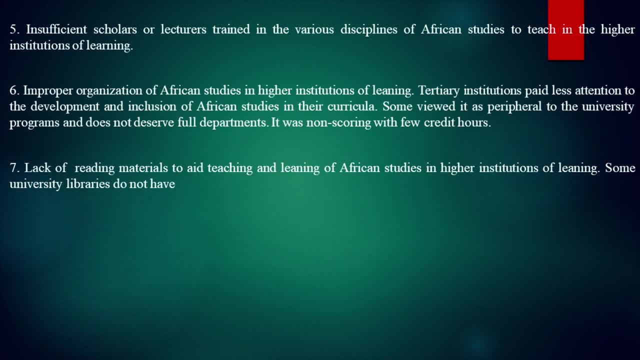 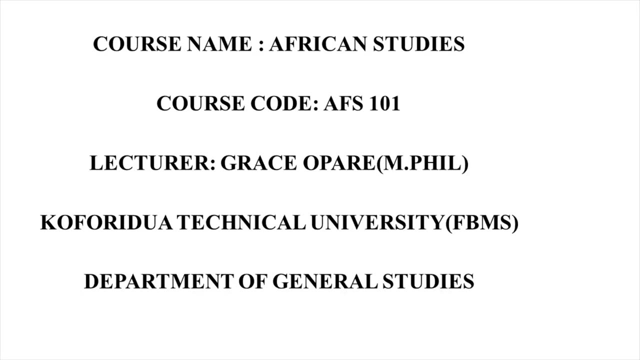 with inferior minds. at the end of the lecture, we indicated that some of these misconceptions are untrue. others are true, but they are not peculiar to the African continent. it is therefore inaccurate for anyone to tag African with such derogatory names where they said and done. let's move into today's 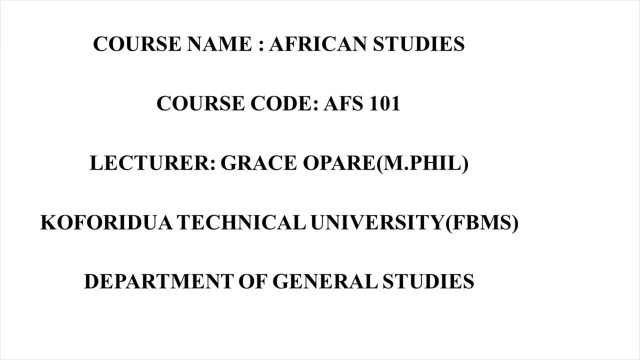 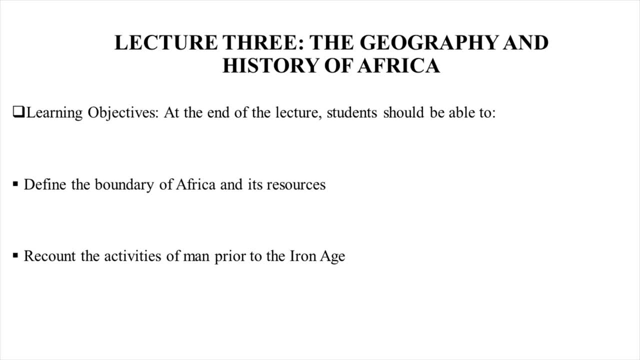 lecture. today is the third lecture, and today our focus is going to be on the geography and the history of Africa. this is African Studies, and so we are going to introduce you to the continent of Africa. At the end of the lecture, you should be able to define. 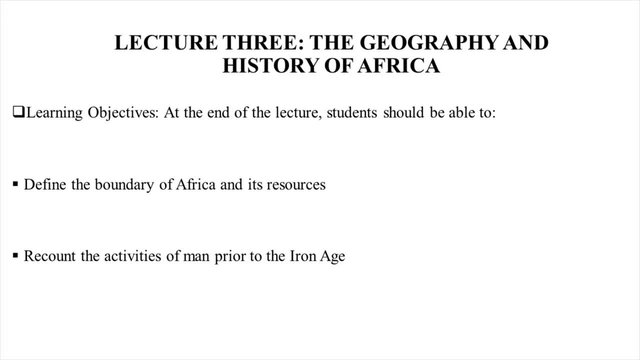 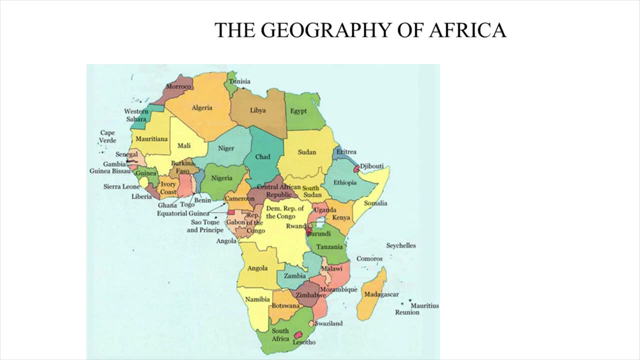 the boundary and then the resources that are found in Africa. You should also be able to recount the activities of Africans prior to the Iron Age. On your screen, you will find the African map. What you see is the map of Africa Among the various continents in the world. 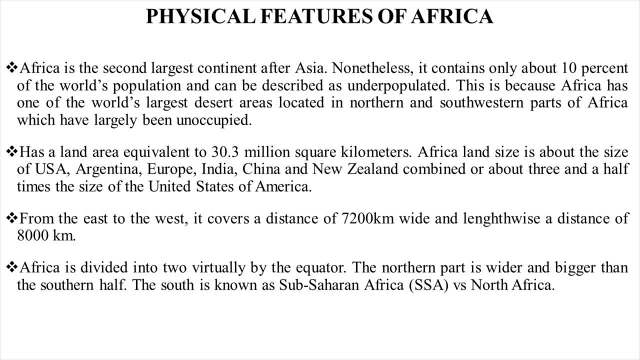 Africa is known to be the second largest continent after Asia. This means that the only continent in the world that is bigger than Africa is Asia. In spite of Africa being the second largest continent in the world, its population, when it is calculated in terms of the world's population, is just. 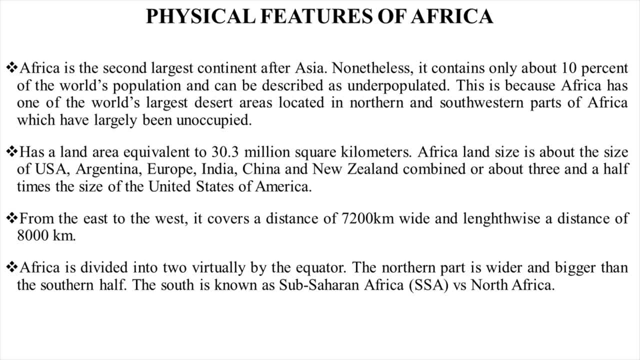 10% of the world's population. Because of this, one can say that Africa is a continent that is underpopulated, because the size of the continent does not match with the number of people living in it. This is given to the reason that in Africa, 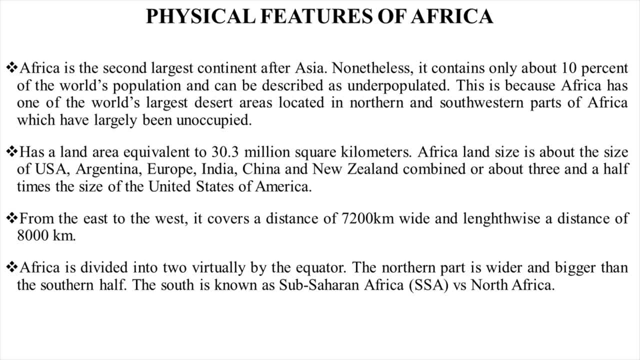 you find one of the world's largest desert areas, that is, the Sahara Desert, located right in Africa. This implies that there is a very large land area in Africa which is unhabitable where you find that there are no people living in that area. 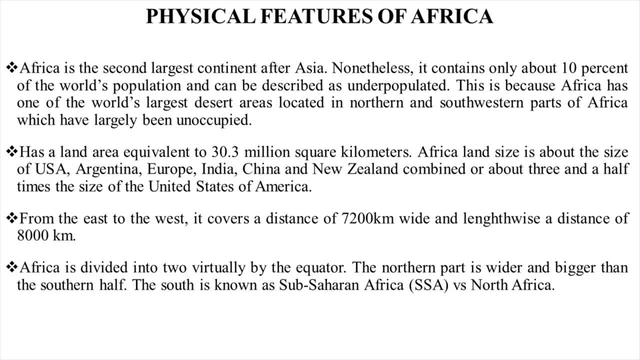 This is because the conditions of the desert area does not make the place suitable to be inhabited by human beings, even animals and even plants. Because of this, even though Africa is the second largest continent in the world, it makes up only 10% of the world's population. 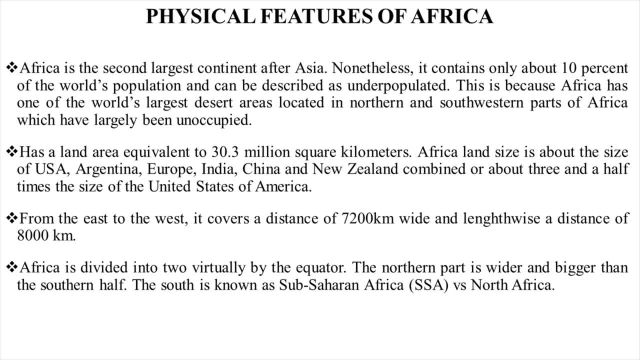 If you want to look at the land area of Africa in terms of its square kilometers, the size of Africa is 30.3 million square kilometers. If you want to calculate the size in terms of countries, you can say that the size of Africa is equal to a combination of the size of the United States of America. 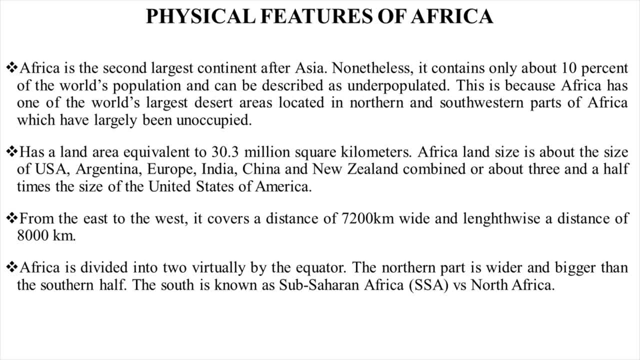 Argentina, Europe, India, China and New Zealand. That is, when you put the sizes of all these countries together, then you can find the size of Africa. From the east to the west, the distance of Africa is about 30. It is about 7,200 kilometers wide. 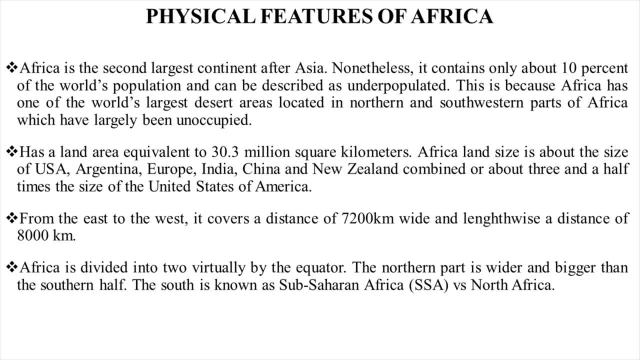 And then when you look at the length, that is, from the north to the south, you find a distance of 8,000 kilometers. The equator divides Africa virtually into two parts or into two halves, So we have the northern Africa and then the south Africa or the southern parts of Africa. 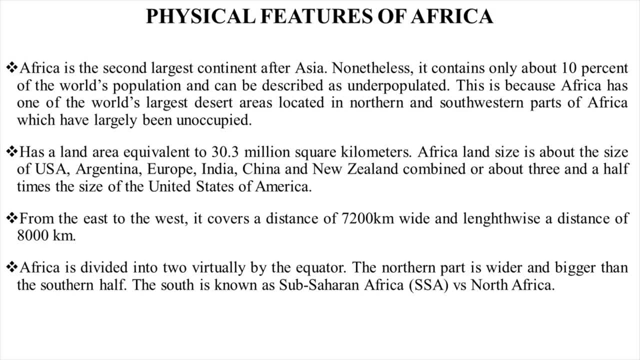 The southern part of Africa is what is referred to as the southern part of Africa. The southern part of Africa is what is referred to as the southern part of Africa. So we have the northern part of Africa and the southern part of Africa. The northern part of Africa was invaded by the Arabs. 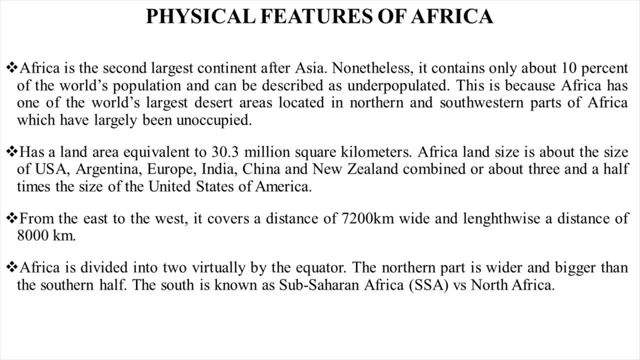 Because of this, you find most of the countries in this area to be practices or believers of the Islam faith. And then you come to the southern part of Africa. it is the part which was also invaded by the Europeans and the British, And so you find most of their population to be Christians. 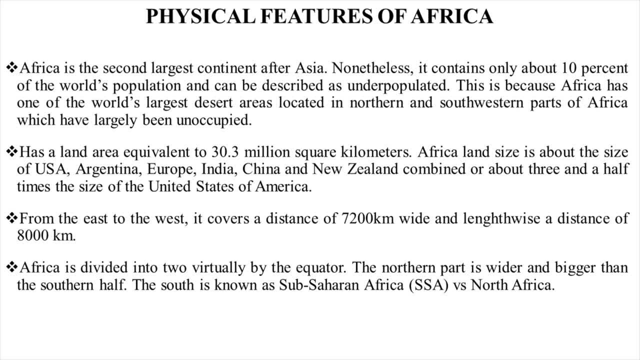 And so you find most of their population to be Christians. most of the people living in North Africa are fair-skinned, That is, they are fair in completion. And then you have people living in the Southern Africa or Sub-Saharan Africa as the dark-skinned or dark in completion. 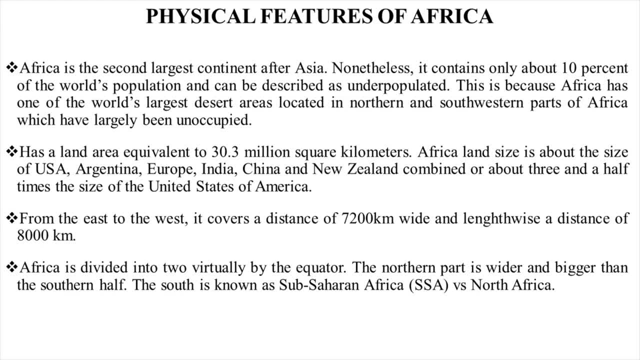 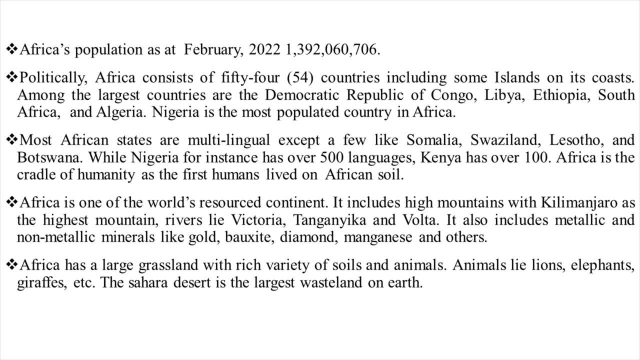 Because of this, it's incorrect to define an African by the color of his or her skin, because you find both fair and dark completion people living in the continent of Africa. As of February 2022, the population of Africa is 1,392,060,706.. 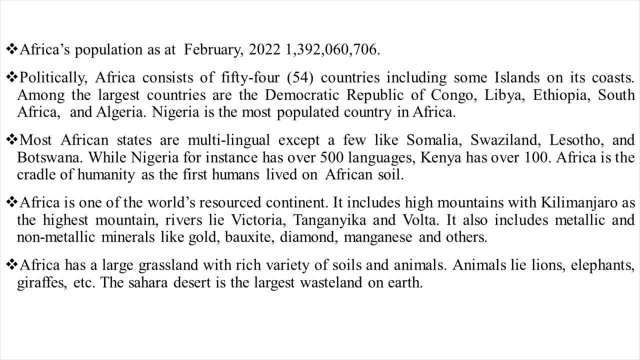 Africa consists of 54 countries, including islands on its coast and the Pacific Ocean, And then countries on its land areas. Madagascar, which is one of the biggest islands in the world, is located in Africa. You find other islands like the Seychelles and Comoros. 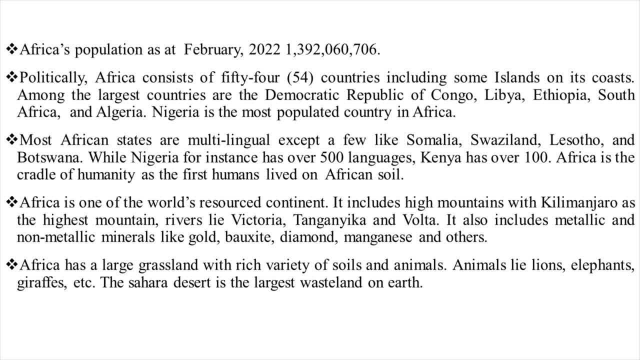 Sao Tome. They all make up the 54 countries in Africa. When you come to Africa, you find that Africa is one of the most important countries in the world. You can see that most of the states or the countries are multilingual. This means that the African people 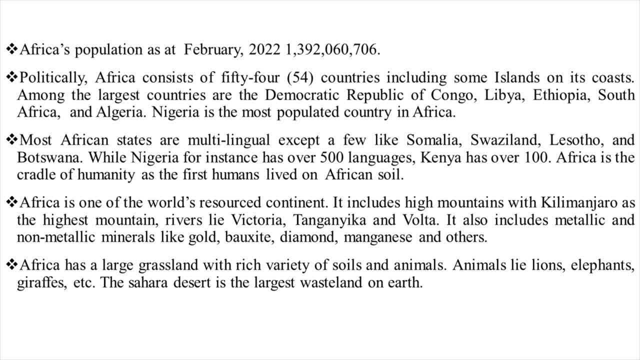 speak several different languages. This implies that you cannot pinpoint one particular language and ascribe it to the African people. You cannot say that in Africa they speak this language, like you will say about, but the United Kingdom, Unless you want to divide Africa into Anglophone or Francophone countries. 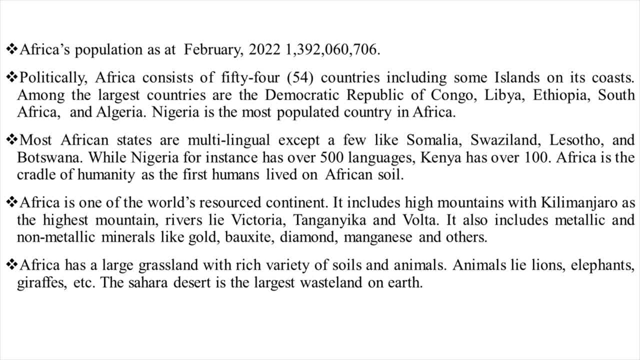 then you can say that this part of Africa has an official language which is French, or an official language which is English. But traditionally the African states, or Africa as a continent, is a multilingual continent. In Africa the African people speak English. 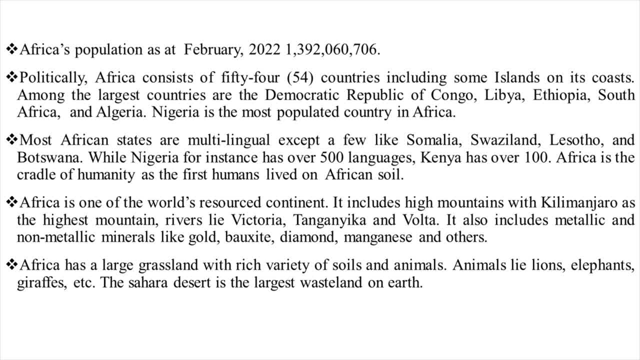 In Nigeria alone, for instance, you find more than or around 500 languages. When you come to Kenya, there is about 100 or even more different languages that are spoken in that country alone. Ghana also has over more than 40 languages that are spoken in the country. 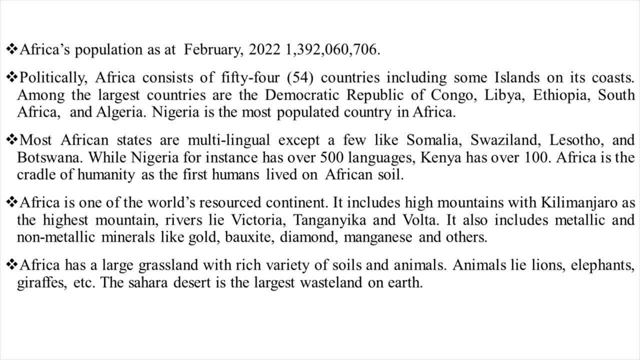 I would want to emphasize that Africa has more than 40 languages. I would want to emphasize that Africa has more than 40 languages. Africa is a continent and not a country. it is a continent with 54 different countries. Africa is known to be one of the world's resource continents and in 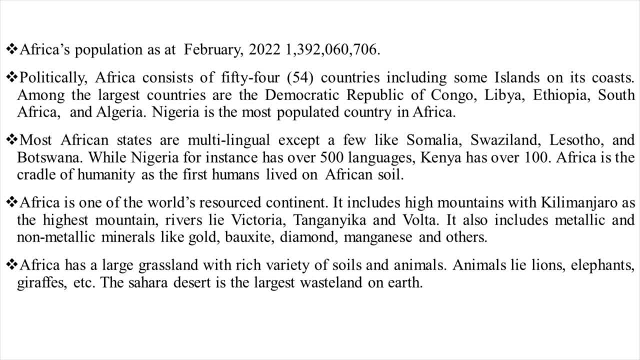 terms of resources. the greater part of Africans resources are natural resources, and so, when you come to Africa, you find minerals like gold, bursites, manganese, fossil fuel. there are large vegetations of grasslands, wildlife like the elephants, you have the hippopotamus, the lion, we have large river bodies, mountains. 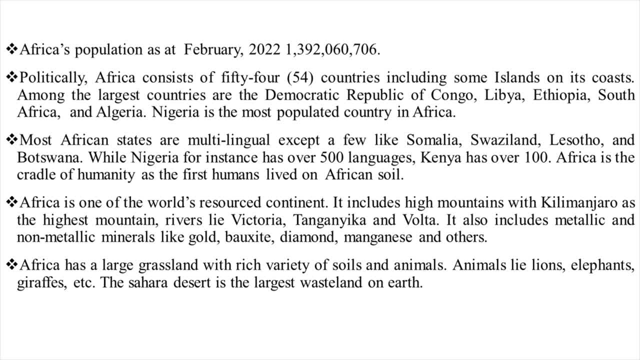 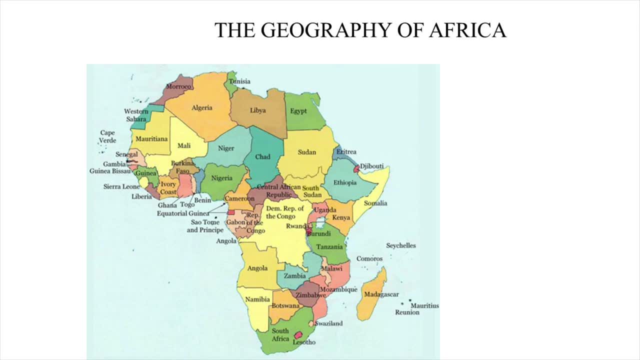 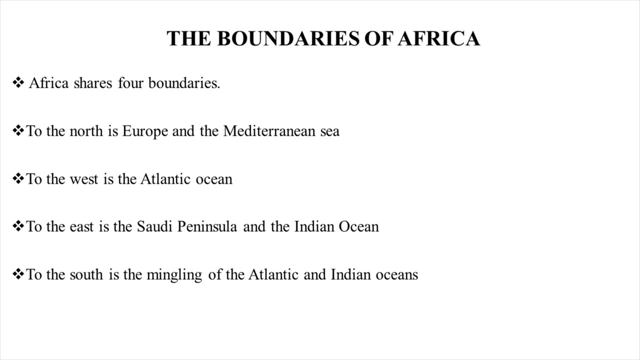 timber and a whole lot. Africa is indeed a very well-resourced continent and its resources are largely natural. let's go back to the map of Africa. Africa has four boundaries and to the north it shares boundaries with Europe in the Mediterranean Sea. to the West is the Atlantic Ocean. the eastern part of Africa shares boundaries with a. 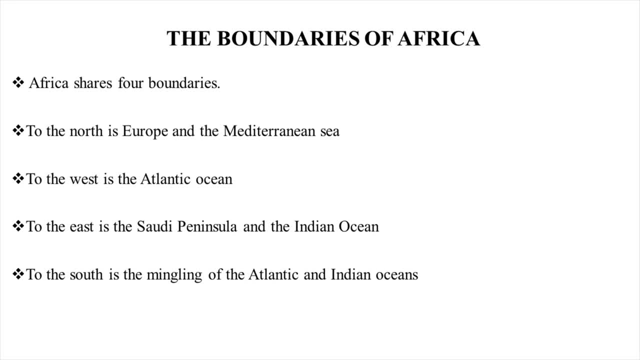 Saudi Peninsula and the Indian Ocean to the south is a mixture of the Indian Ocean and the Atlantic Ocean. if you look at the four boundaries of Africa, one can say that Africa shares boundaries largely with the ocean. most of Africa's boundaries are the Atlantic and the Indian Ocean. let's look at the history of Africa. 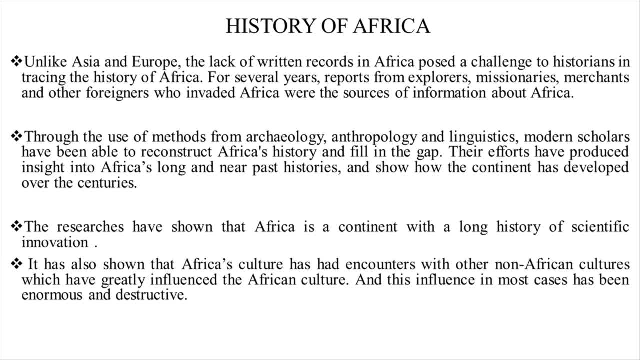 unlike Asia and Europe and other continents, Africa as a continent, originally large written record of its history, some early Europeans and non Africans were of the view that Africa did not have a history for several years. what the African knew about him or herself and what non Africans knew about the African. 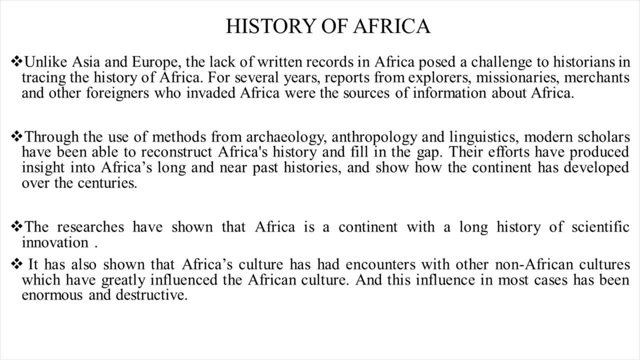 continent and the African people were report from early European explorers and missionaries who visited the continent of Africa. but through the use of modern methods from our education, now some Africans and some and even some Europeans, through archaeological findings, anthropology and linguistics or studies in linguistics, are able or have been able to recount and reconstruct the. 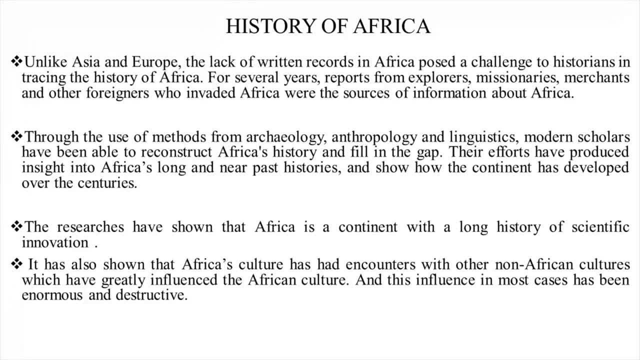 history of the continent of Africa and the African people. because of this, one can say that there is a history of Africa and a history of the African people. this construction by the African scholars, or modern scholars, indicates that Africa, as a continent, has had a history full of scientific innovation. its history had 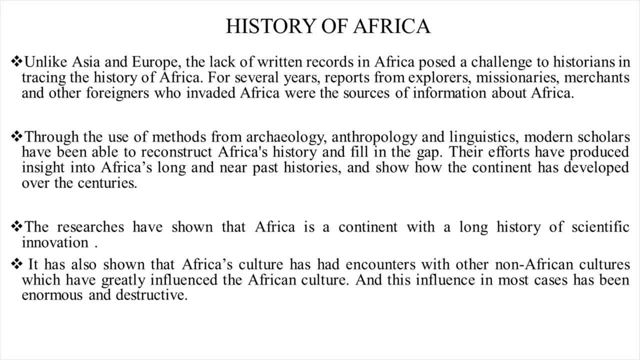 had contacts with several other cultures and these other cultures have had immense influence on the cultures of Africa. because of this, one can say that the history and the culture of the African people has evolved and developed over the years. it has not remained static but has changed as pus or times also changed and as Africa got into contact. 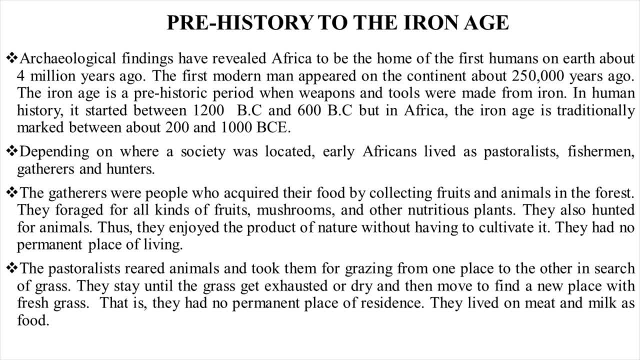 with other cultures. let's look at pre-history to the Iron Age in human history. Some studies have given three time periods in human history: the Bronze Age, the Stone Age and the Iron Age. The Stone Age is seen as the period in human history where human beings or where humans made tools or weapons from stones or by the use of stones. 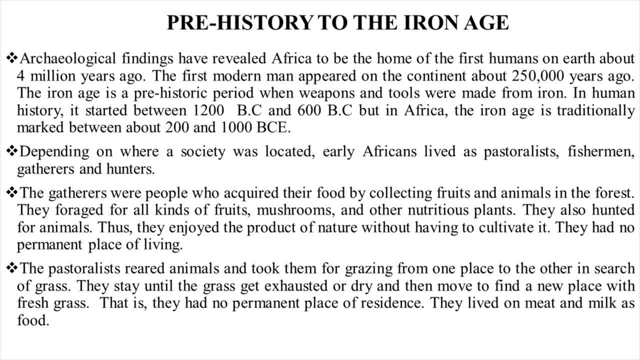 Several years later, the metal known as bronze was discovered, So humans began to use bronze in the manufacturing of tools and weapons in their daily activities, And this period is referred to as the Bronze Age. After the Bronze Age was the discovery of iron. 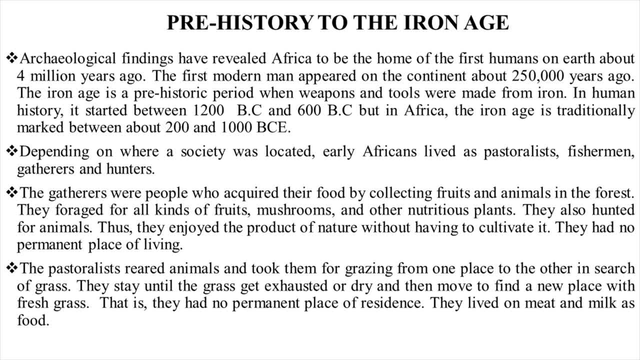 And this marks the period of the Iron Age. So the Iron Age is. This is seen as the period in human history where human beings used iron in the manufacturing of tools and other weapons which helped in their daily activities In Africa, or before the Iron Age. archaeological findings have revealed that Africa is the first place to be inhabited or to be inhabited by human beings. 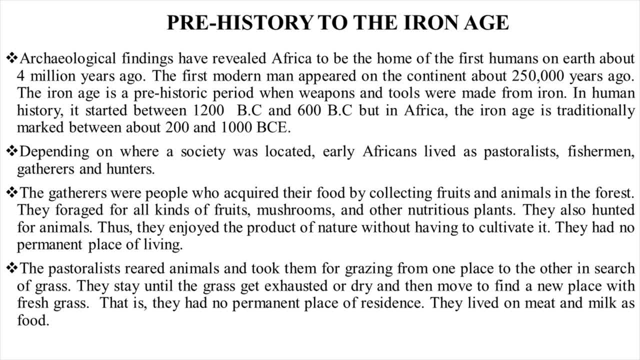 Research shows that. Research shows that It was the first place human beings lived before they migrated to other parts or they moved to other parts of the world about four million years ago. The first modern man research has shown is said to have appeared on the continent of Africa about 250,000 years ago. 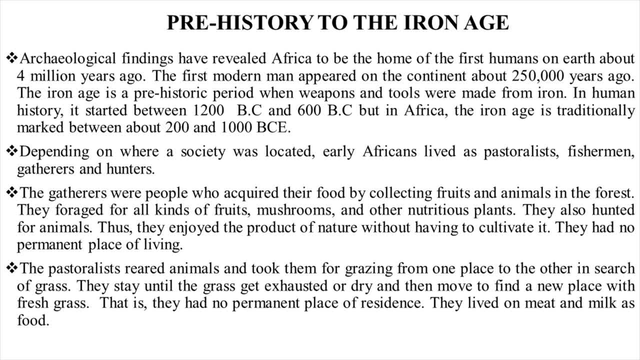 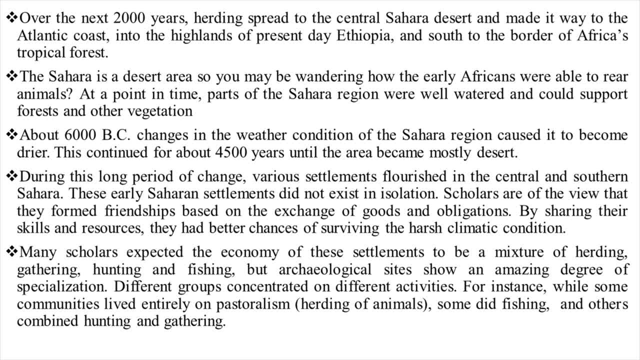 each other to the extent that there were a mixture of activities. but research shows that, even though the people had adopted some new behaviors from each other, there was evidence to show that the people largely specialized in their own traditional economic activities. this means that the pastoralist were still practicing the rearing of animals, the guardrails were still going into the forest, 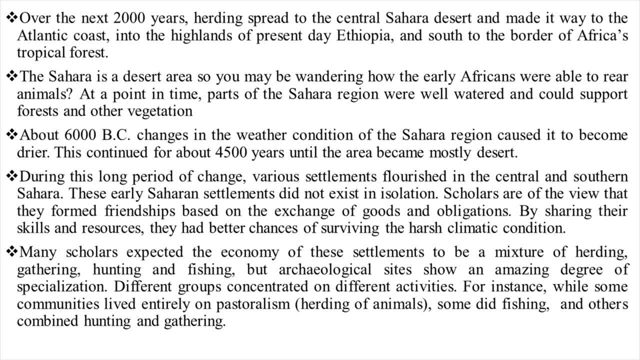 to gather their food to feed themselves, same with the fishermen and the hunters. however, they adapted new ways of living or borrowed behaviors from each other. as the climate continued to change in the sahara area and the area began to get dry, it could not provide for the new settlers. 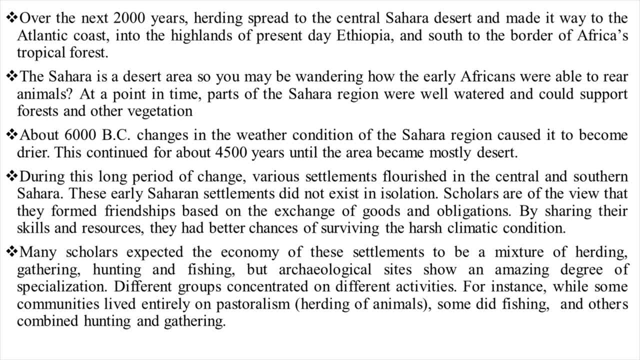 what they needed to survive on. the grasses were drying up so the pastoralists could not get enough grasses for their animals to graze or for their animals to feed. their place was drying up, so when the guardrails go into the forest they were not getting. 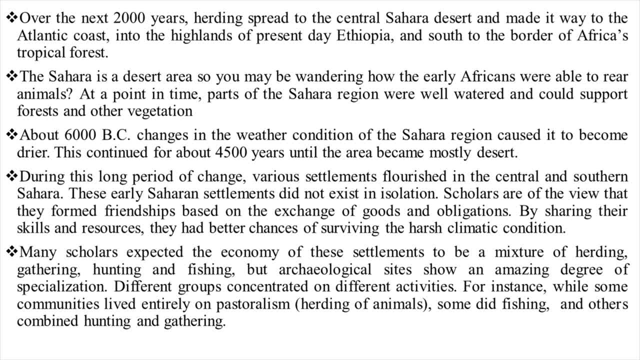 enough food to feed themselves. in their families, same with the fishermen and the hunters, they were not getting enough game or enough fishes to live on, so they began to adapt to new ways of living. they began to experiment with their environment. so from that experimentation they began to grow food. 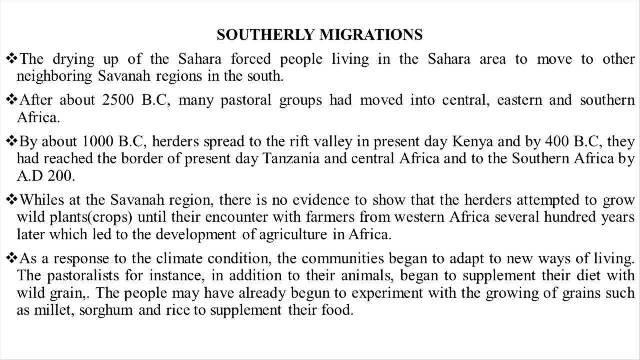 to feed or to supplement their traditional or original food. What this means is that, as time went on, the people living in the Sahara Desert came to know about agriculture, as they came to adopt new ways of living. There is not much evidence to show that the pastoralists and the guardrails 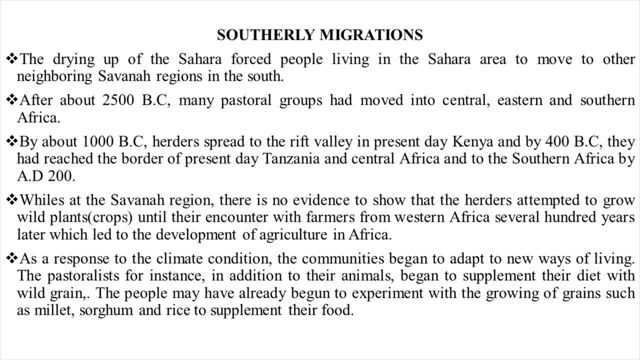 began to cultivate their own food, But there is evidence to show that as they moved from the Sahara region into the Savannah region and they had contact with people living in West Africa, they adopted the practice of cultivating their own food. The West Africans also had as their economic activity agriculture. 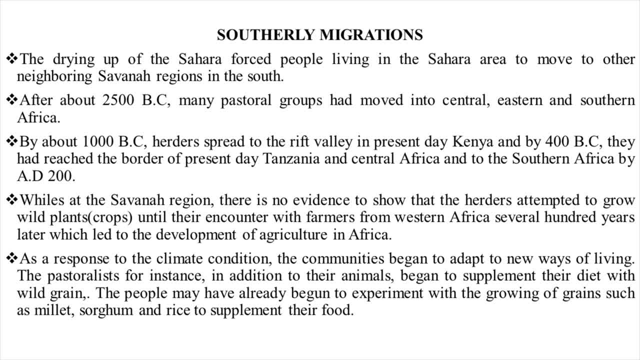 So when the people who migrated from the Savannah region, who migrated from the Sahara area, came into contact with the people living in the Savannah region, they developed the act of farming, or agriculture. So they began to grow crops like, or to grow grains like, wheat. 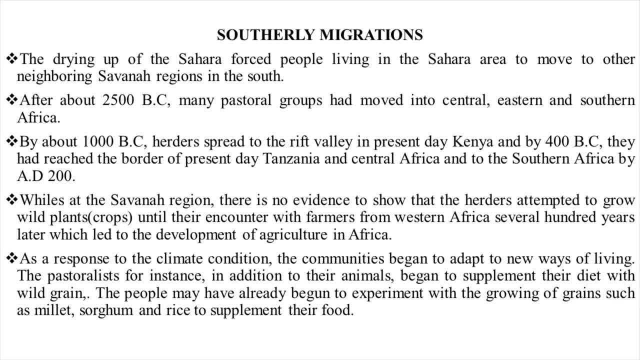 millet, sorghum and rice to supplement their food. But the weather condition did not get better. It continued to change and it continued And it continued to dry things up And this even affected the source of water, or the sources of water for the people. 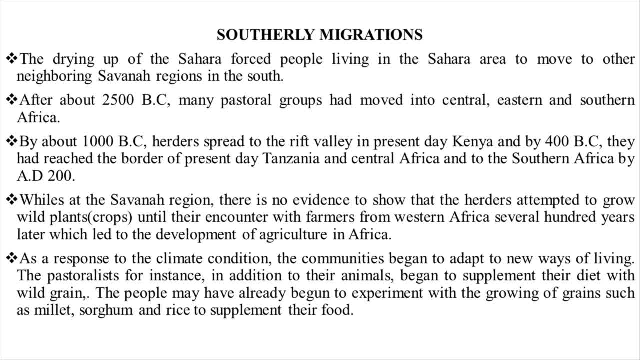 This meant that at a particular point in time, there was scarcity of water where both human beings and animals had to live on the same source or sources of water, And because it was a very difficult time for the people living in the Sahara, it was nearly impossible for animals and then human beings to live on the same sources of water. 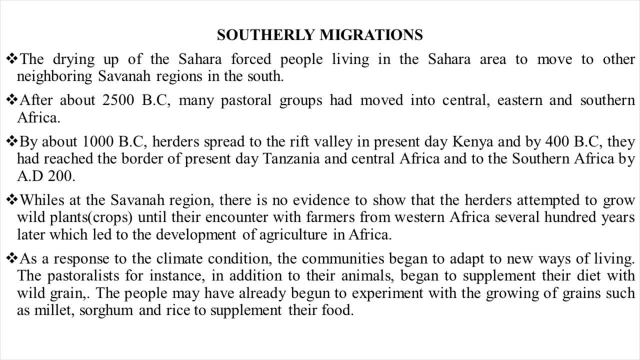 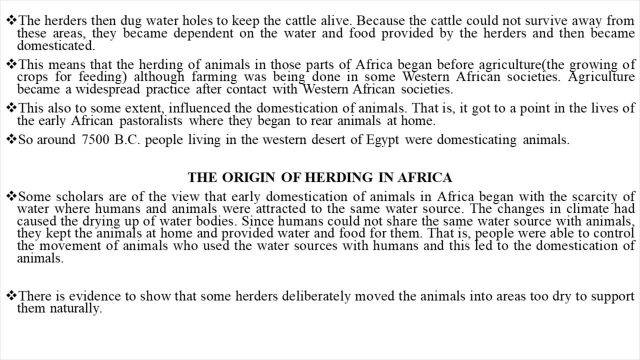 A new activity emerged. Indeed, human beings and animals could not survive on the same sources of water, because the animals were prone to contamination or because the animals were not easy to control. All do the same because of the water. The water takes too long. 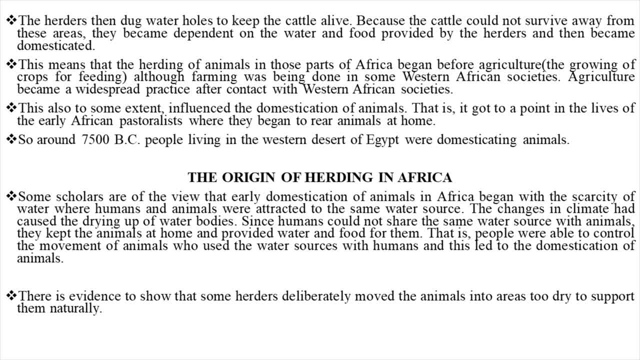 could contaminate the water. whenever animals go into a river source to drink water, there was the likelihood that they will step into the water and get it muddy. they could even ease themselves into the water. they could infect and contaminate the water, which would have had a bad impact on the lives of the humans. so 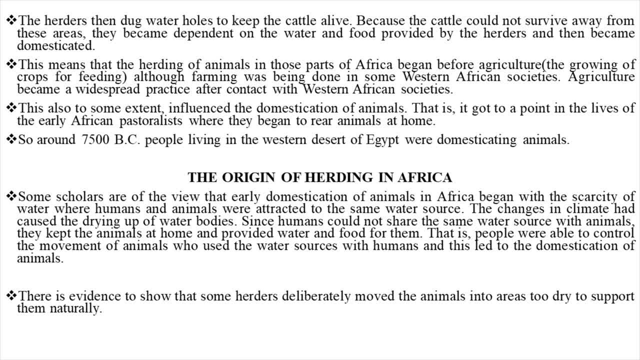 human beings, or at the early Africans, devised a strategy, and this strategy was to keep the animals at home, not necessarily their places of residence, but it could have, but also at places where you could have a place of residence, where you could have a place of residence. so human beings, or at the early Africans, devised a strategy, and this strategy was: 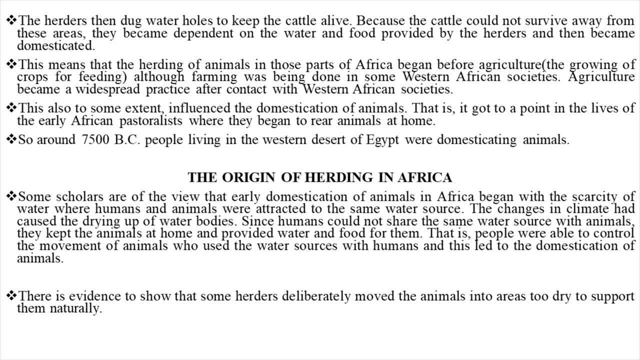 to keep the animals at home, and this gave rise to the domestication of animals in Africa. so here the pastoralist would keep the animals in a pen or find a land area where they can keep them, so they will go into the bush, get the grasses the. 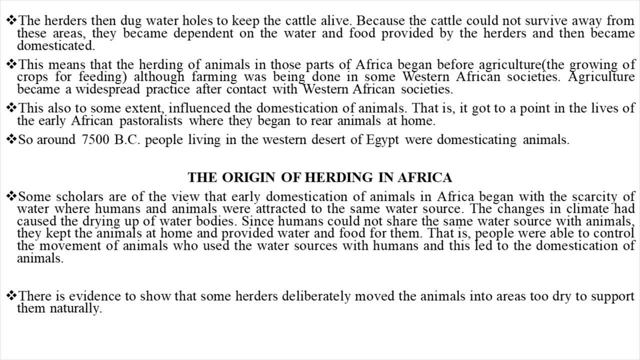 animals need to feed on and then bring in water for the animals, and this was done to protect the water sources that the early Africans were living on. as the practice of keeping the animals at home continued, animals became domesticated in Africa. so when you want to talk about the origin of 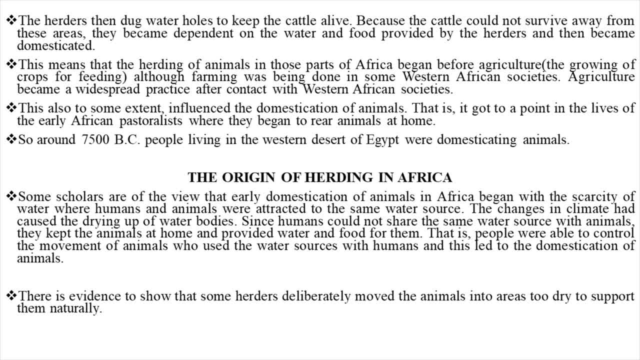 domestication in Africa. one can say that the scarcity of water sources in Africa compelled the early Africans to keep the animals at home and rather provide for them their food and their sources of water. there is evidence to show that some early Africans deliberately took the animals into land areas that did not provide them with the food and 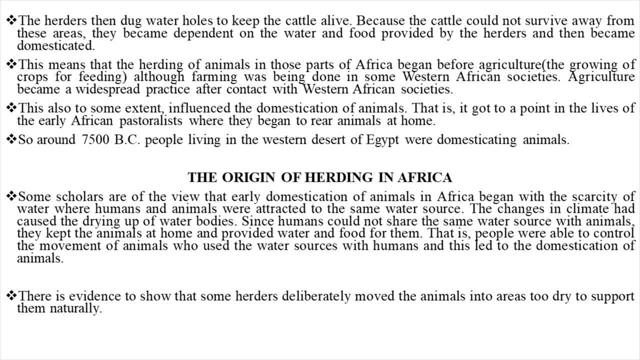 the waterfall. they needed to survive from the old. because of that, the animals stayed at one particular area. what they survived on was what their mustis or what the head is brought to them as food and water. This practice continued until date. We continue to domesticate animals. 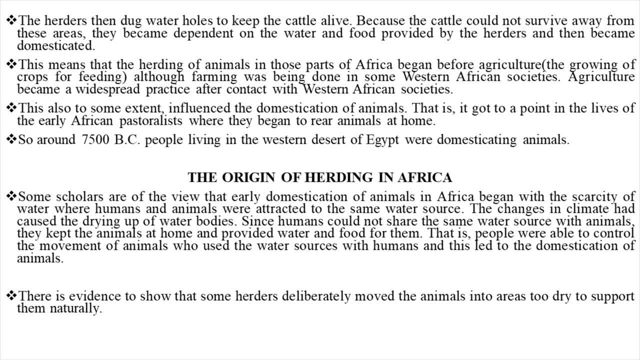 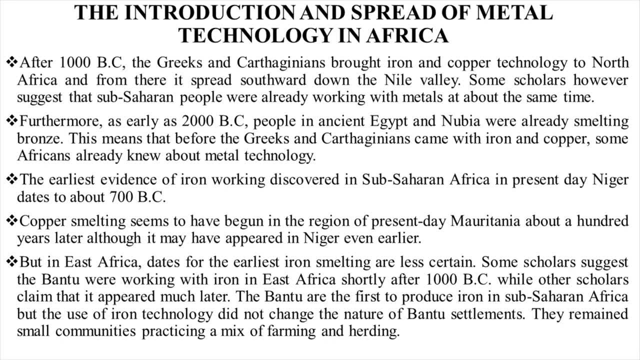 in various or respective countries or societies. Let's look at the introduction and spread of metal technology in Africa Around the year 1000 BC. research shows, or indicates, that the Greeks and the Carthaginians brought iron and copper technology to North Africa. 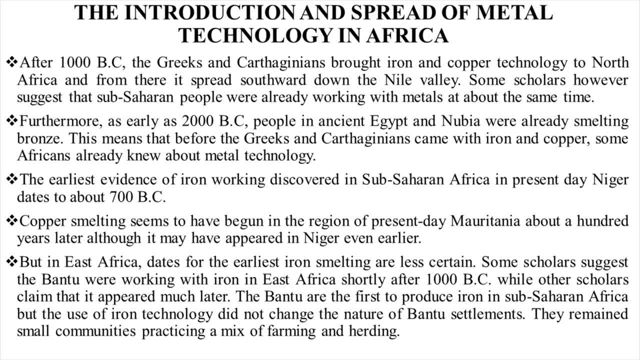 and from there it spread southwards all the way to the Nile Valley. This means that iron technology came to Africa through the Greeks and the Carthaginians. Other studies indicate that even before the Carthaginians and the Greeks brought iron to Africa. 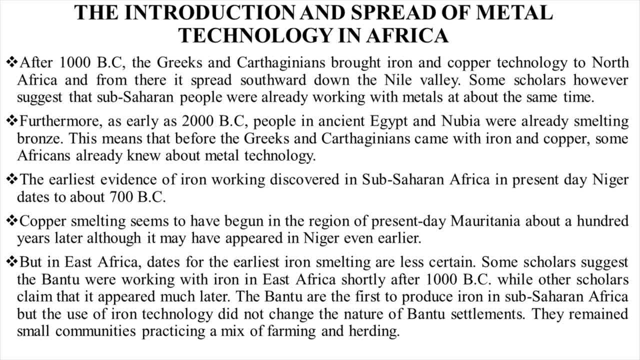 around the same time, that is, around the same 1000 BC, where the Greeks and the Carthaginians brought or introduced iron to Africa. the people in the sub-Sahara Africa region were already working with metals At that same time, again around the year 2000 BC. 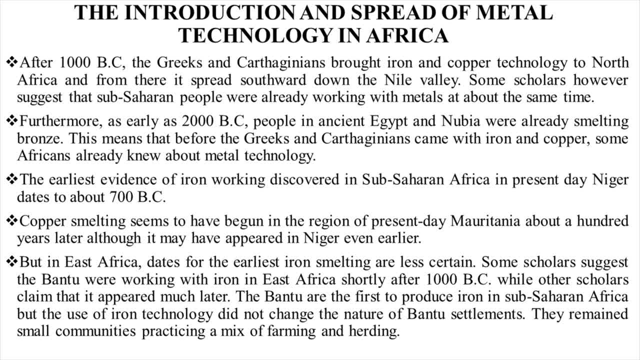 there is evidence to show that people in Egypt, and then the Nubians, were also smelting bronze. This put together suggests that before the Greeks and the Carthaginians introduced iron to the African people, Africans already had knowledge about metal technology. 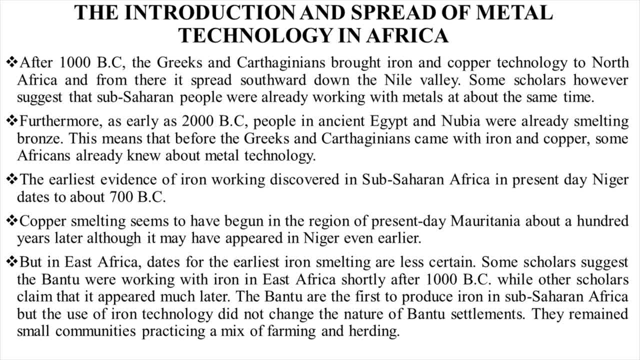 However, this knowledge was not widespread, but was limited to the societies where they were practiced. The introduction of iron by the Greeks and the Carthaginians, rather, gave a widespread nature to metal technology in Africa. If you look at East Africa, research has not been able to. 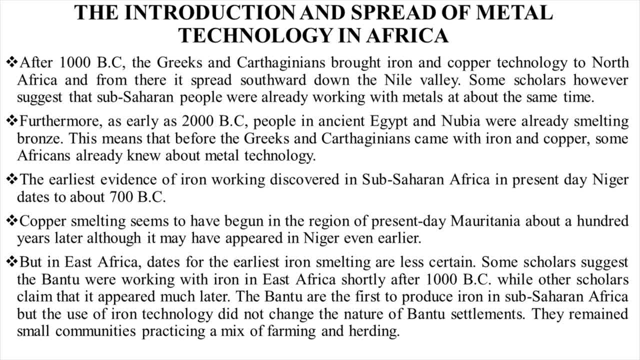 give a definite time period or date where the smelting of iron began. Nonetheless, some scholars suggest that the Bantu people, who are located in South Africa, were working with iron somewhere around 1000 BC. Some scholars even claim that the Bantus working 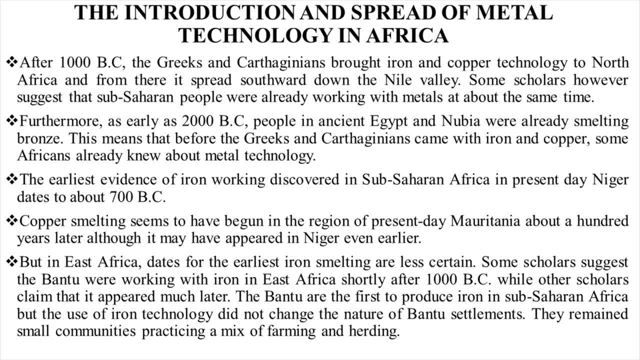 with iron, or some scholars even claim that the Bantus were working with iron even earlier, before 1000 BC. The Bantus are known to be the first people to produce iron in South Sahara Africa, But the use of iron technology did not change. 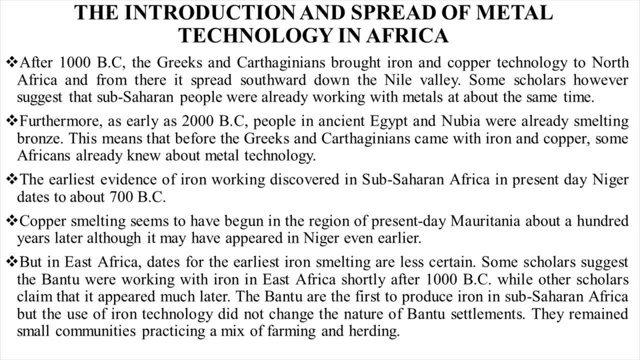 their society or the way the Bantus lived their lives. So when the Africans came to know about metal technology or came to know about iron, research shows that it had an impact on their lives. One of them is that before iron technology, 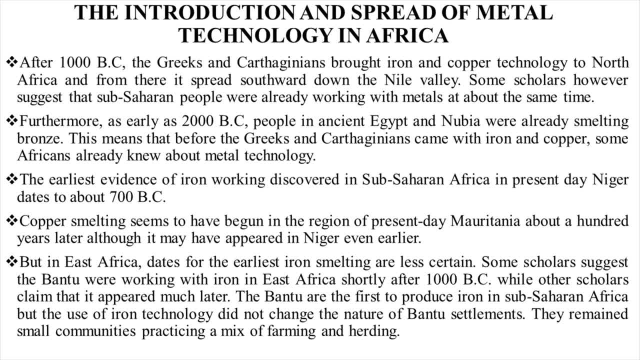 the African, either as a pastoralist undertook its activities with sticks or bones or animal bones. The farmers undertook their farming activities or by clearing land areas with animal bones or sticks, or weapons or tools they produced from stones or other resources in their natural environment. 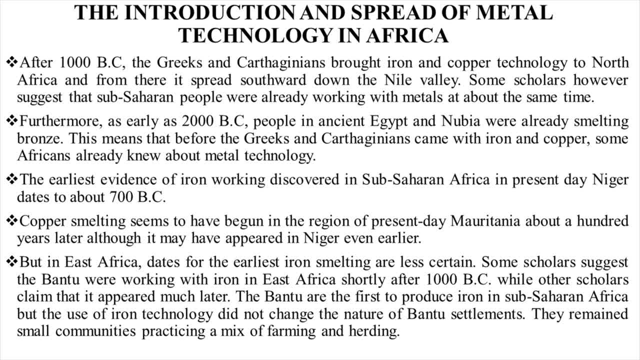 And so when iron was introduced, the African could now smelt the iron and produce farm implements like cutlasses and hoops. This helped them to be able to clear large areas of land much easier and faster for their farming activities. So the introduction of iron, 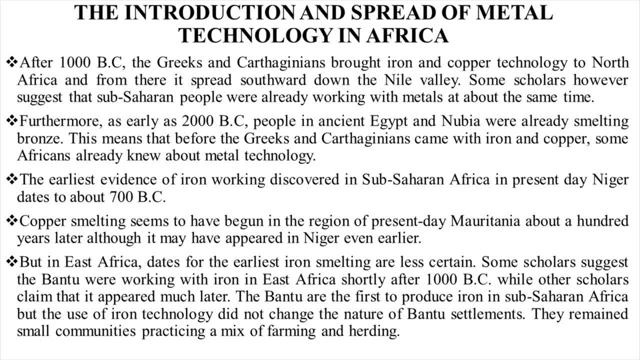 contributed to the production of farm farming tools, which aided in the agricultural activities of early Africans. Again, it allowed the early Africans to move into new areas, clear them and make their own settlements So people living in a particular area could find a new place. 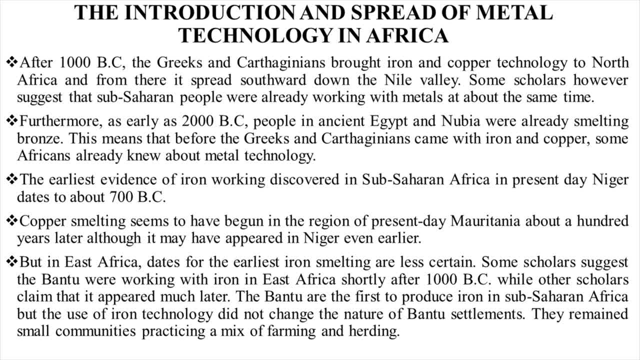 move and settle there. Because of that, the settlements or the land area of the African people was increasing. People were now not living in clusters. Rather, they could move into even far places to settle, And this collectively expanded the settlements of the early Africans. 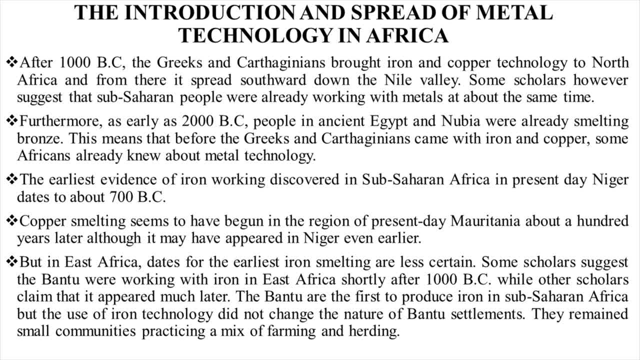 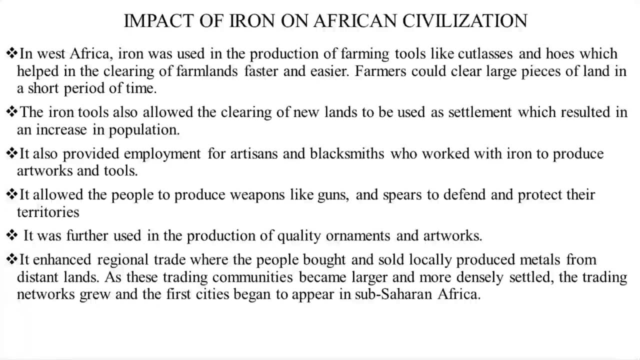 So new areas or new settlements were developing or were emerging, And this led to an increase in the population of African Africa. It also provided employment for the artisans- The blacksmiths and the artisans who were working with stones, and the blacksmiths could. 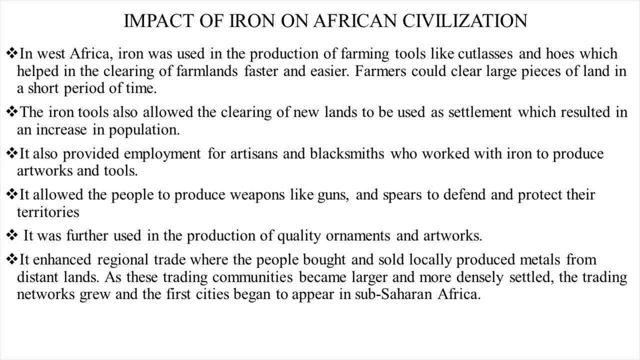 now smelt the iron and produce tools and weapons and implements for people. People were paying them for the production of these artworks. People were also paying them for the production of the tools At that particular moment in time, because iron or metal technology was new in Africa. 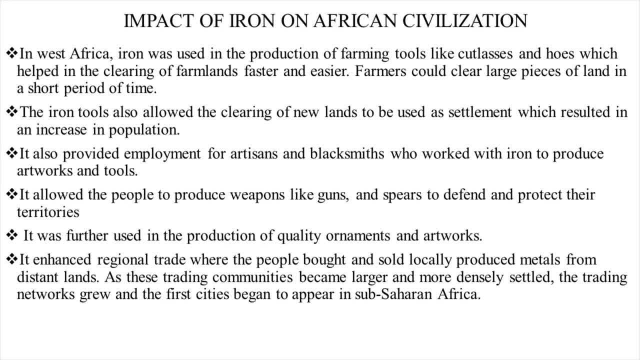 the people who were into its production- the blacksmiths, the artisans- became very important people in society. It gave them money, it gave them power and then it gave them authority. It also allowed the early Africans to produce weapons from iron. 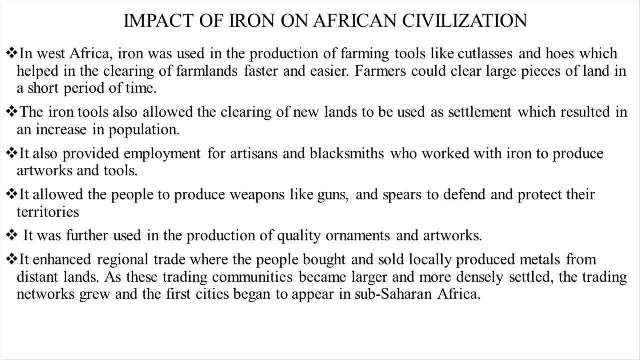 They could now produce guns and spears and bow and arrow which they could use to protect their territories and to defend themselves. Furthermore, you can talk about the production of ornaments and artworks. So the impact of the introduction of iron was that it allowed the early 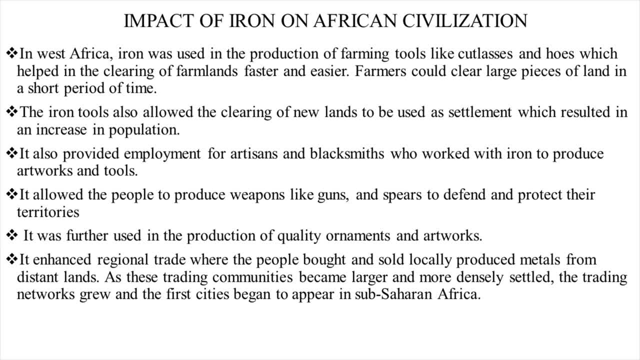 Africans to make beautiful ornaments and artworks to adorn themselves and portray their culture as well. Lastly, it enhanced the regional trade within the savannah region and the sub-Sahara region. People could now trade in metals. People could now trade in the farm tools. 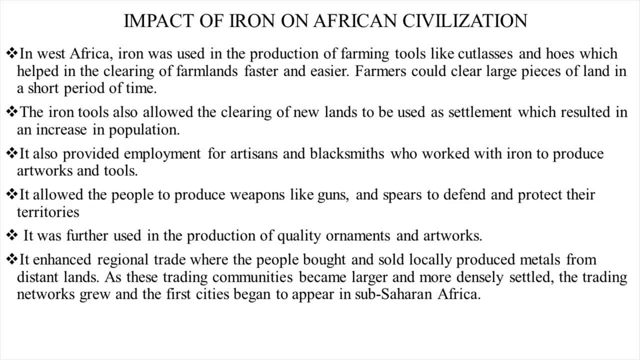 in distant places. So people in sub-Sahara Africa would buy the tools or farming implements or the metal tools from the artisans, travel to distant land areas to sell them to other places, to sell them to other people in other places. It also increased.